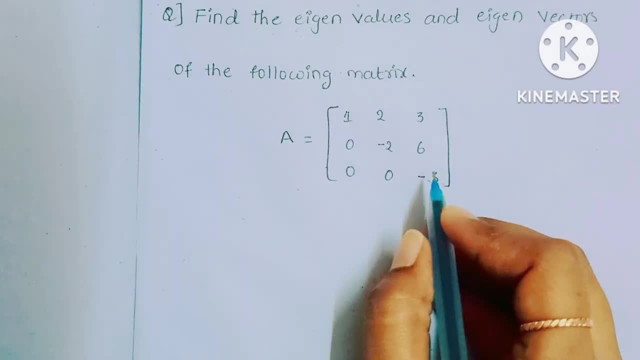 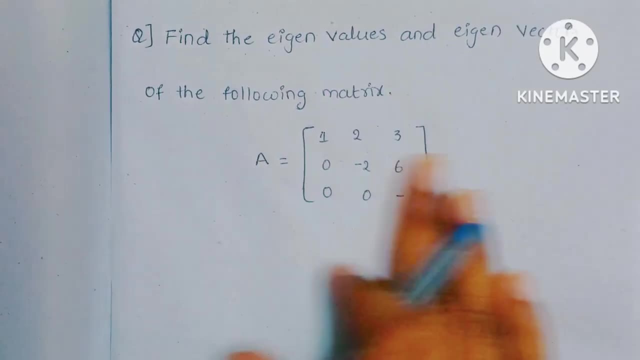 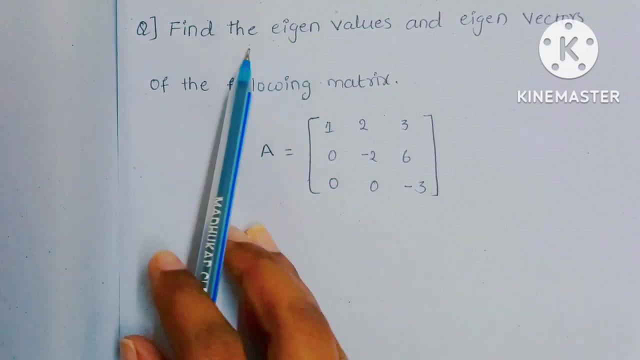 Hi friends, welcome to my channel, NMLM courses with Nagmani. Today I am going to solve a problem on eigenvalues and eigenvectors and I will give some tips during solving this problem. So don't skip the video and watch till the end. If you have any doubt, please comment below and please continue the video. 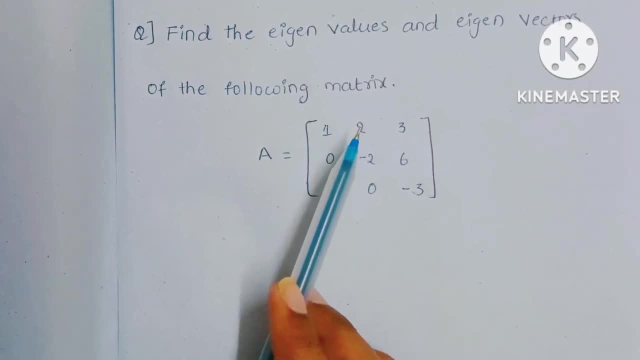 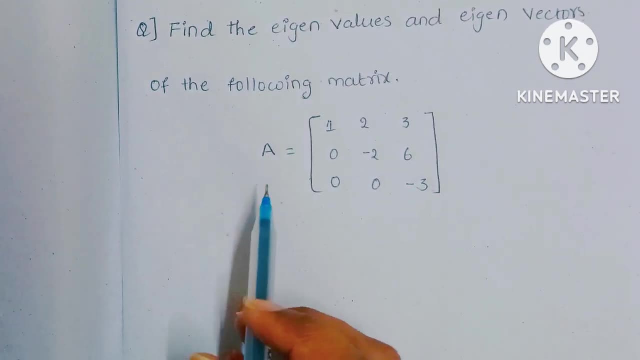 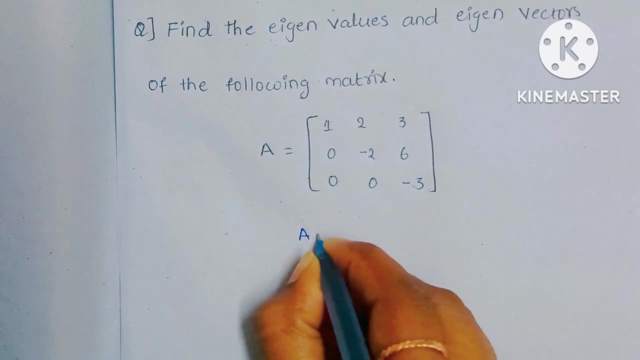 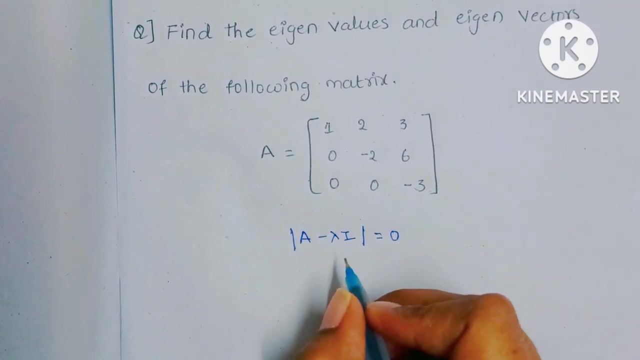 So let's see this problem. This is also upper triangular problem. We will see how to find the eigenvalues and eigenvectors for given matrix. Okay, first, for finding eigenvalues, we have to write characteristic equation that is a minus modulus of a minus lambda i, which is equal to zero. This is the characteristic equation for the given matrix. Okay, here. 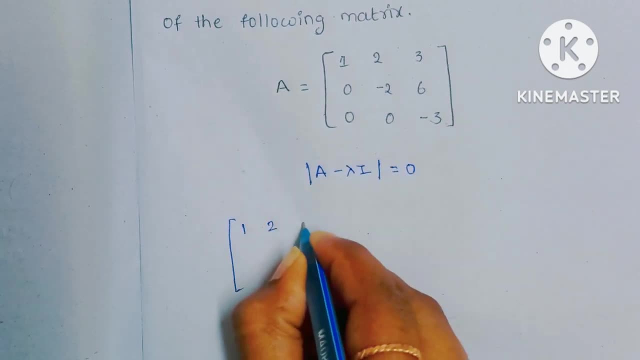 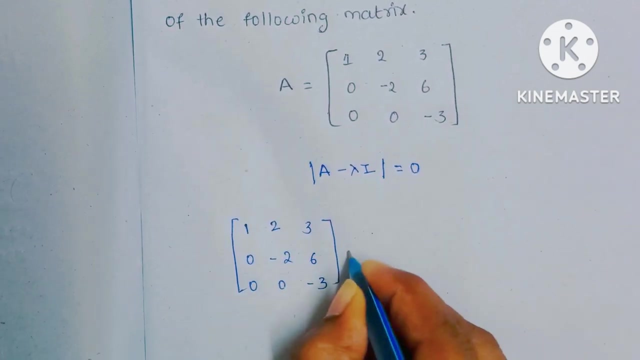 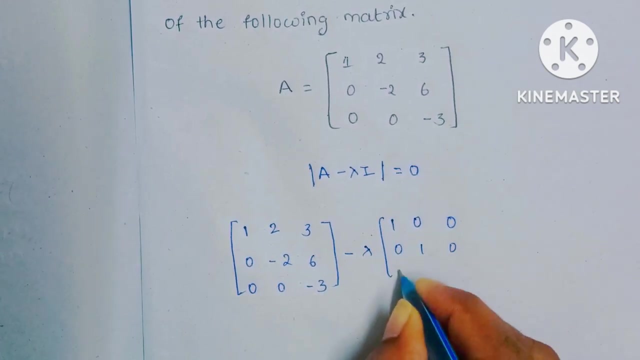 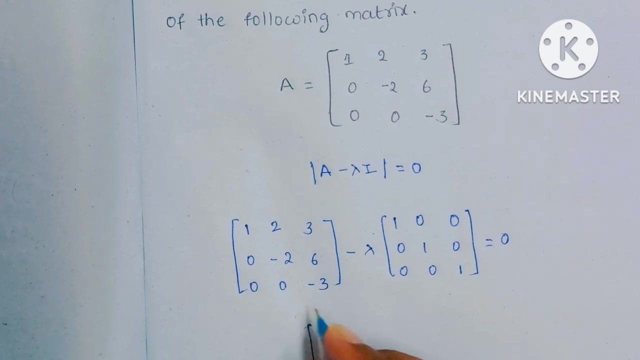 A matrix is 1, 2,, 3, 0, minus 2,, 6,, 0, 0, minus 3 and minus lambda into i is not nothing but identity matrix: 1, 0, 0, 0, 1, 0, 0, 0, 1, which is equal to 0. Okay, here so modulus of this one, and here a minus lambda i. 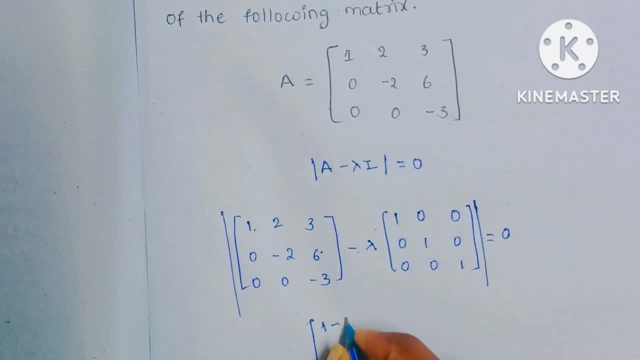 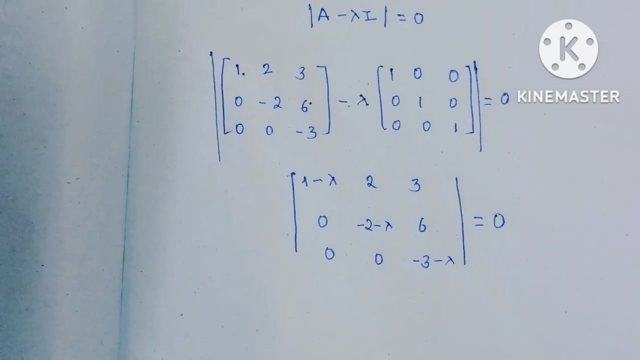 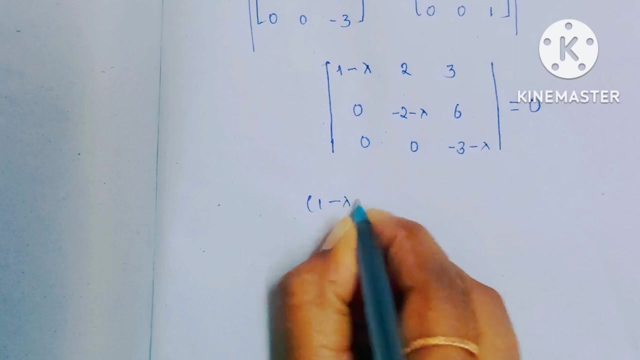 Okay, 1 minus lambda into 1, 1. so 2, 3, 0 here minus 2 minus lambda. and here 6, 0, 0 minus 3 minus lambda, which is equal to 0, sorry, 0. okay, here 1 minus lambda into minus 2 minus lambda into minus 3. 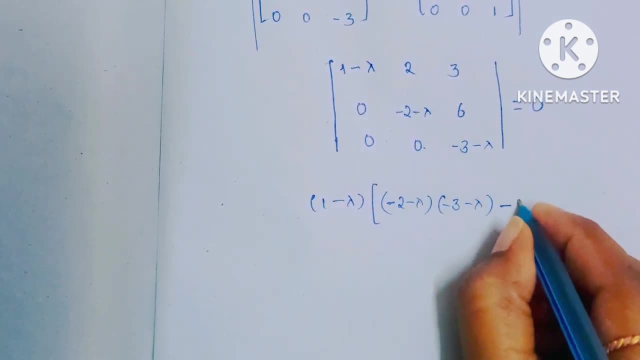 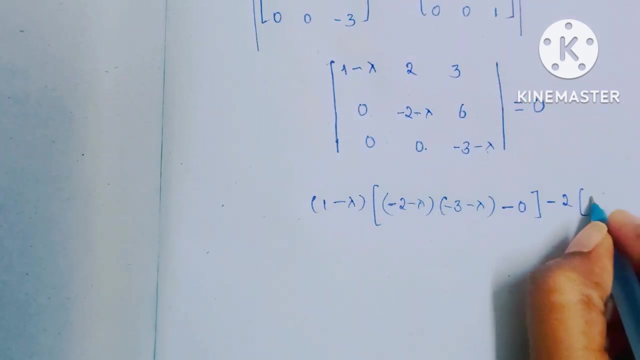 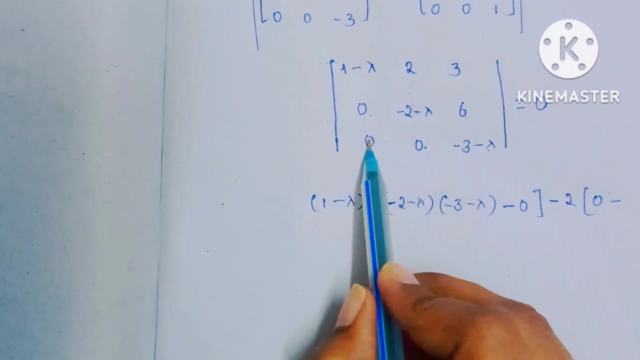 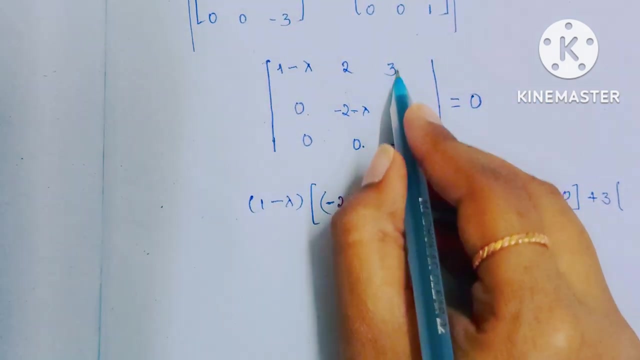 minus lambda minus 0 into 6, 0 minus 2 into here, 0 into something 0 minus. if you close this row and this column, we get 0 into something 0 minus 0 into 6: 0 place 3 into here if you close this column and this row. 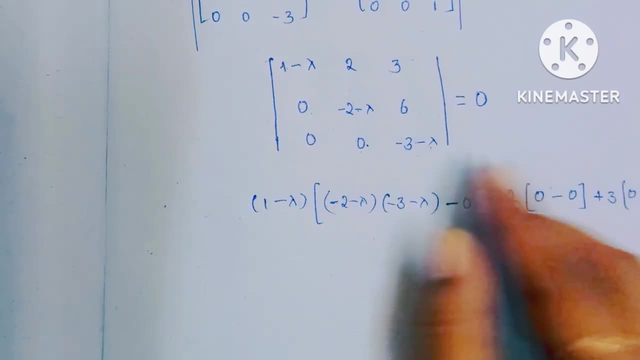 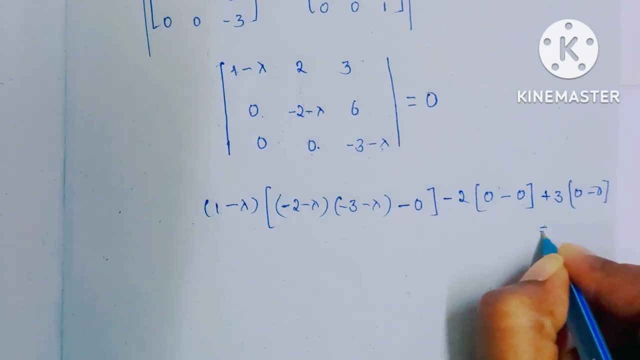 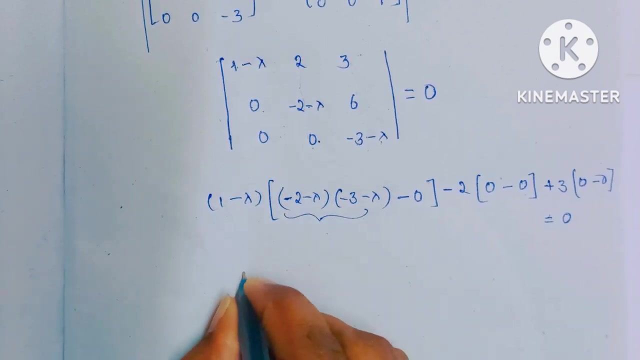 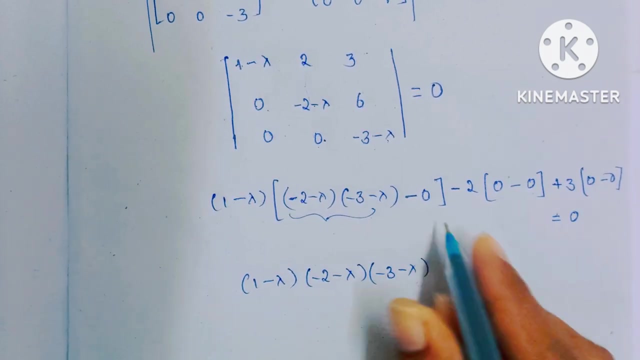 we'll get 0 my into 0, 0 minus 0 into something, 0, okay, okay, which is equal to 0 if you calculate this here when minus lambda into this one. so 1 minus lambda into minus 2 minus lambda, minus 3 minus lambda, 1 minus lambda into. 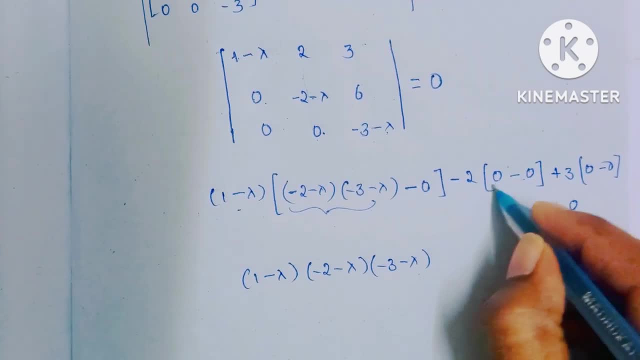 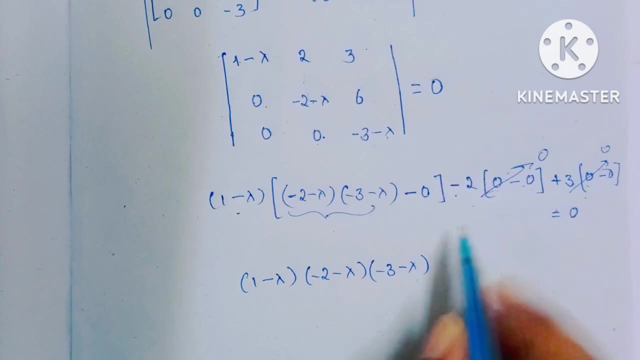 0, 0, so here minus 2 into 0, minus 0 is 0, so 0 into something 0, 0. minus 0, 0, 0 into something 0, so these two terms get cancelled. so here we. this thing is remaining. 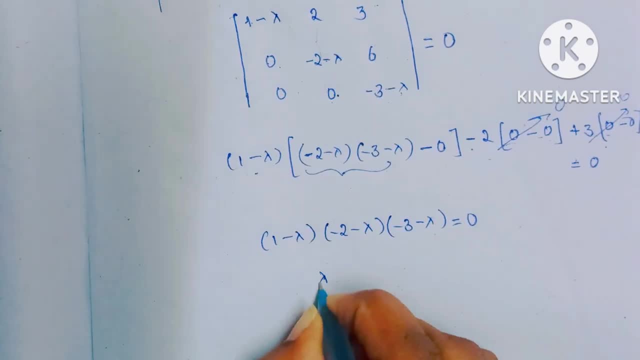 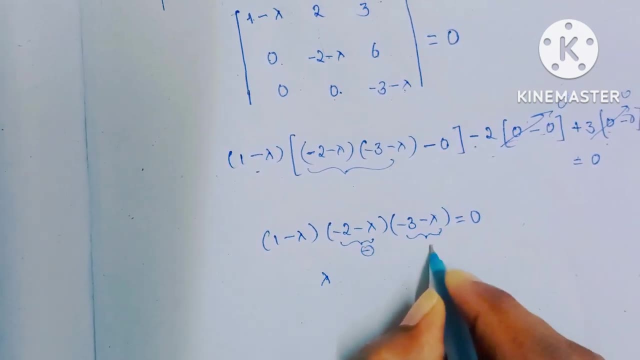 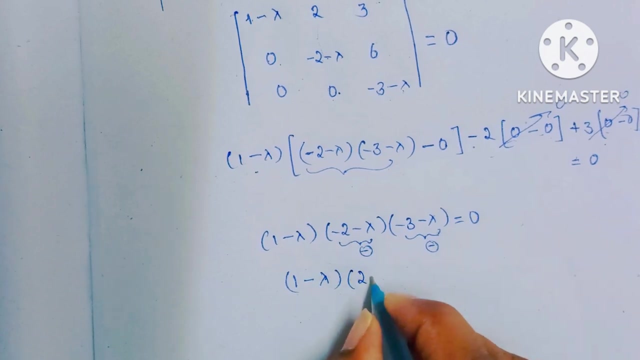 So from this here we can write that lambda equal to: here we can take minus common, here also minus common. So here 1 minus minus, so minus into minus plus. So we can write this equation as 1 minus lambda into: if you take minus common, then 2 plus lambda, here 3 plus lambda, which is equal to 0. 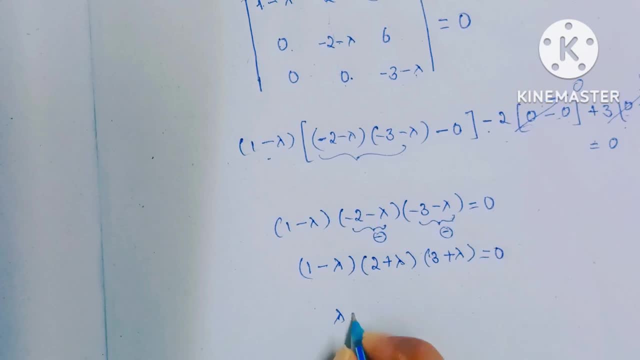 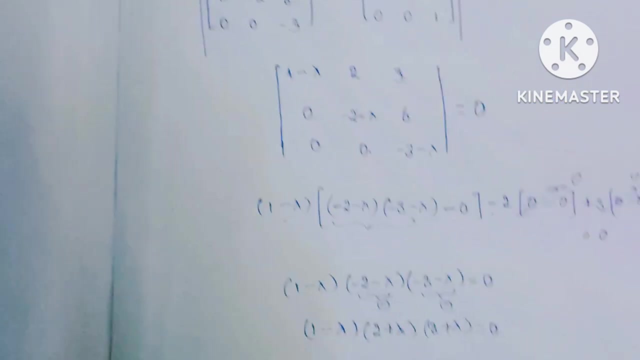 So from this equation we can write: lambda equal to 1, lambda equal to minus 2. here lambda equal to minus 3.. These are the eigenvalues for a given matrix. And if I want to say one trick, that here this is the upper triangular matrix. 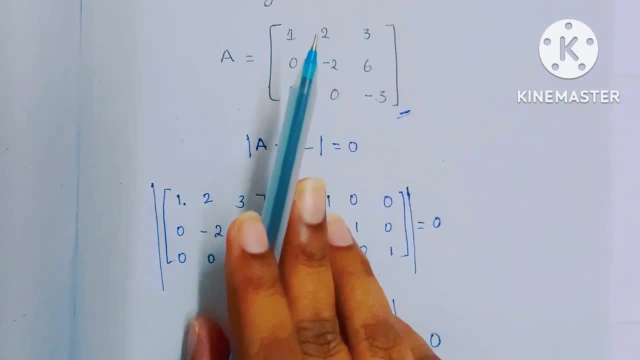 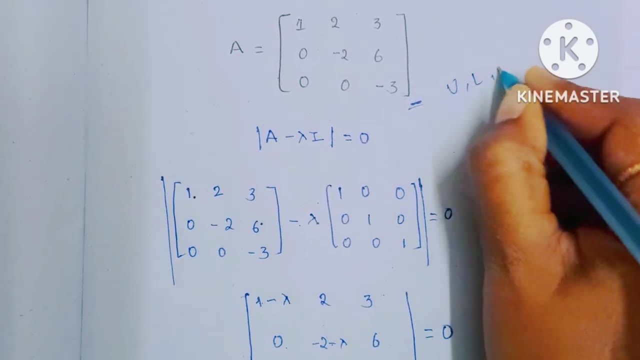 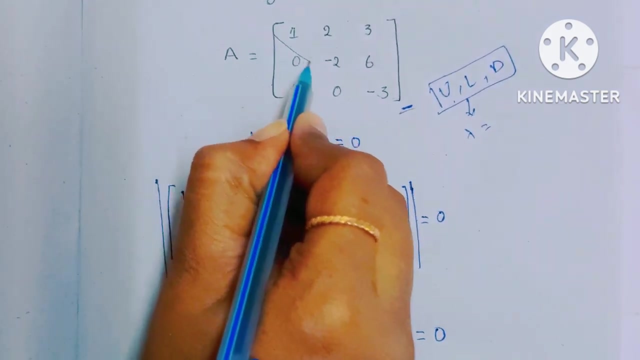 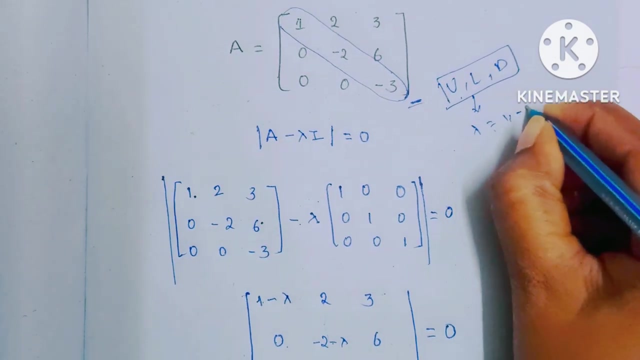 So for a upper triangular matrix or lower triangular matrix or a diagonal matrix, For any upper triangular or lower triangular or diagonal matrix, for these three matrices the eigenvalues are the. whatever the principal diagonal elements are there, that are the eigenvalues. So here, 1 minus 2 minus 3 are the principal diagonal elements. 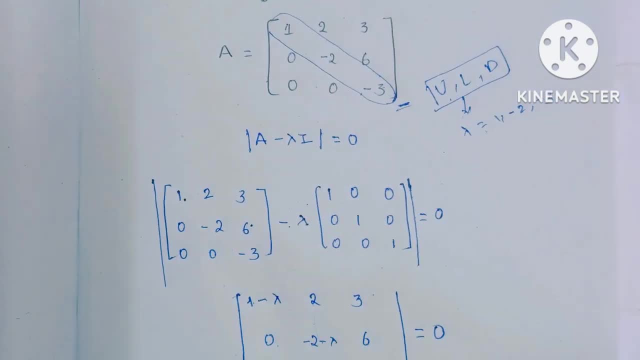 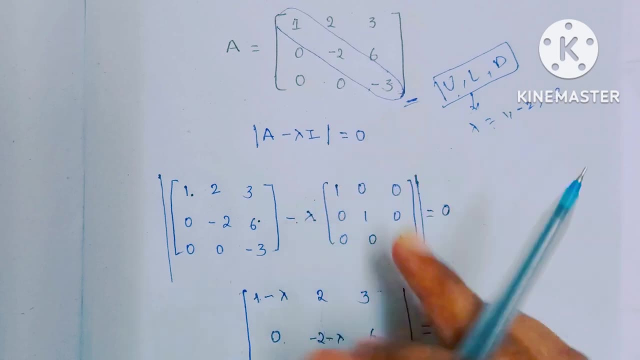 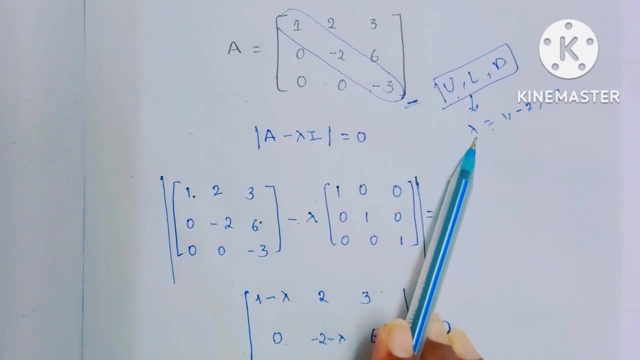 These are the eigenvalues for the given matrix. This, if you see the. these are the. this is one of the property for the Eigenvalues and eigenvectors. So this is the upper triangular. for this, the principal diagonal elements are the Eigenvalues for the upper triangular matrix. 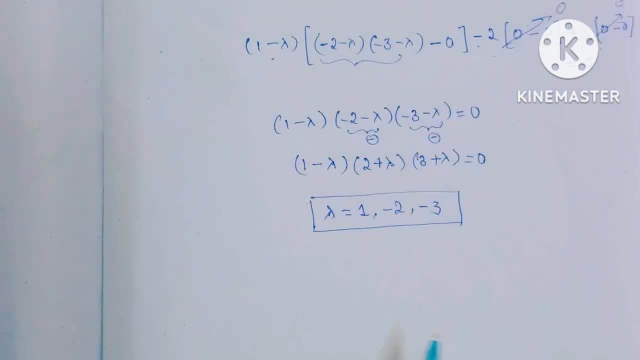 So 1 minus 2 minus 3.. So we also got lambda equal to 1 minus 2 minus 3.. From this we can verify that, whether we got the correct eigenvalues or not. Okay, next we have to find the eigenvectors. 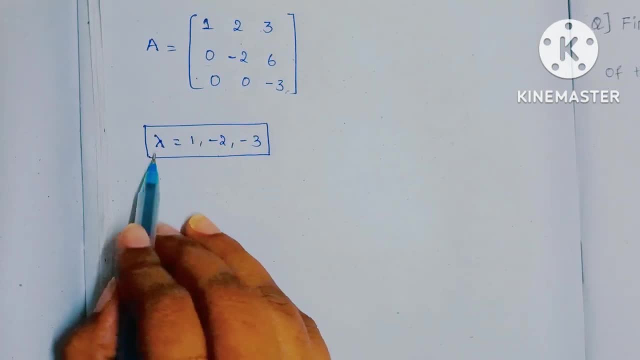 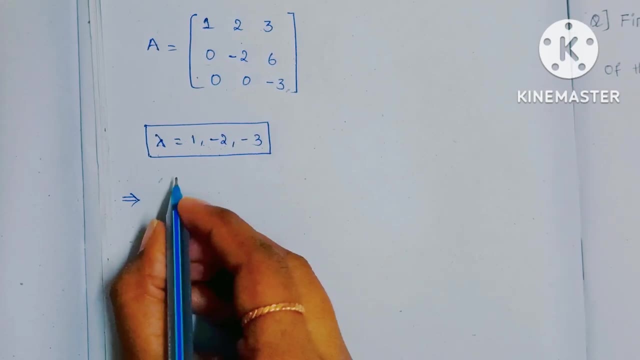 Now here I wrote the given matrix A and the eigenvalues, and from here we know that the eigenvalues are 1 minus 2 minus 3.. So for a eigenvalue lambda equal to 1, we have to find the eigenvectors. 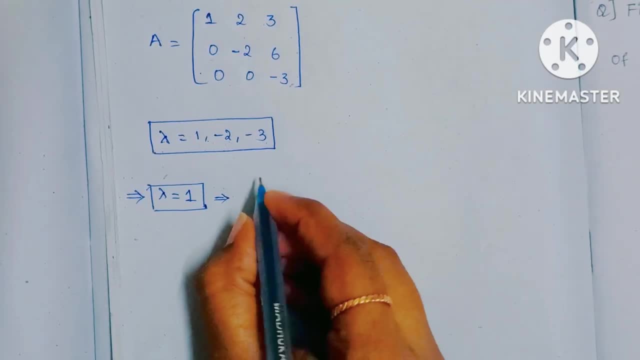 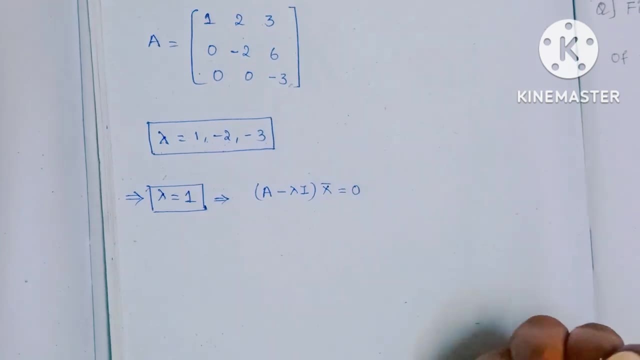 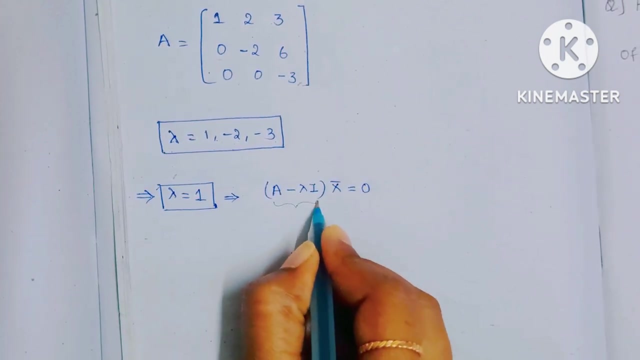 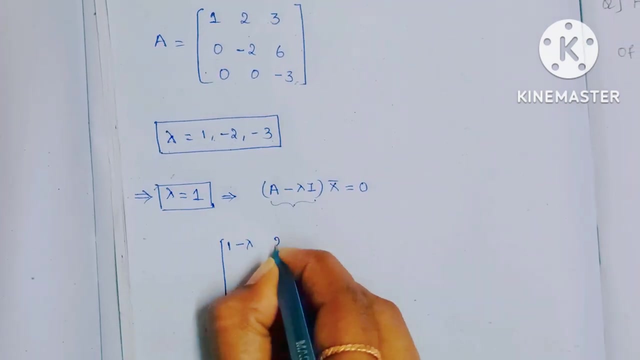 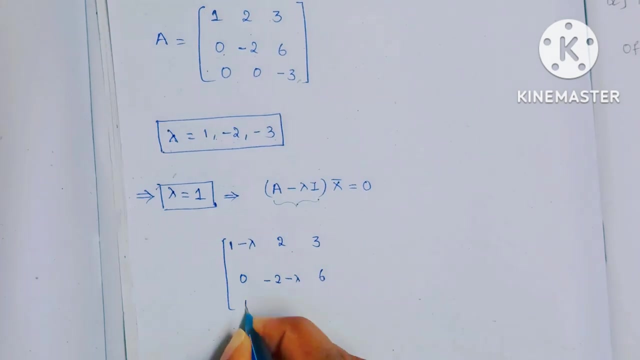 We know the equation for the equation to find the eigenvector, that is a minus lambda i into x bar, which is equal to 0. So here a is The this matrix. so I am directly writing a minus lambda i matrix here: Okay, see 1 minus lambda 2, 3. so here 0 minus 2 minus lambda, here 6: 0, 0 minus 3 minus lambda. 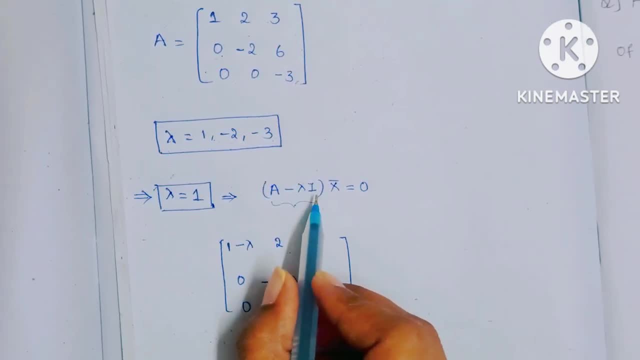 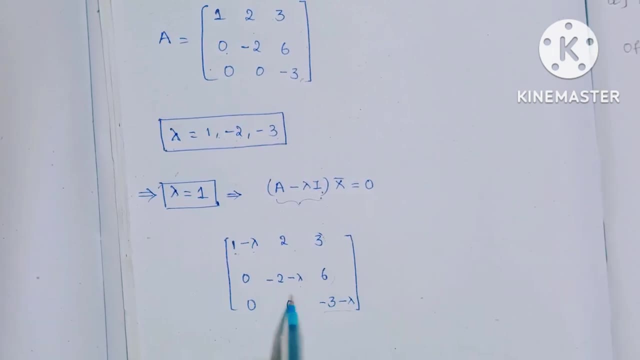 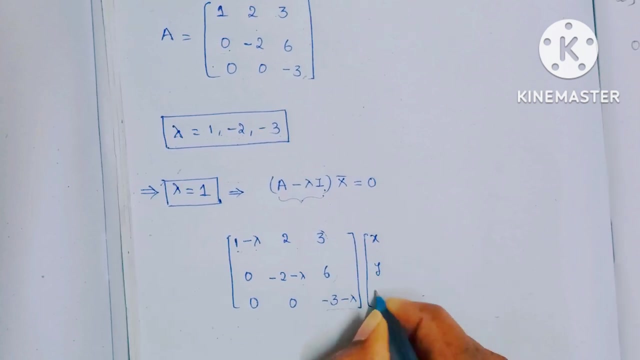 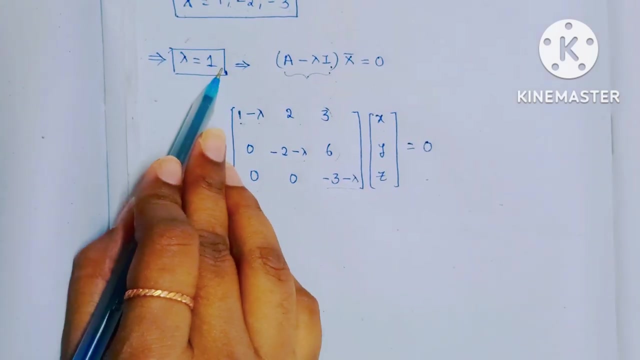 So identity matrix means only the diagonal elements are present now, so directly we only diagonal elements will be changed, and Other Things numbers will be same. so I am writing like this: and here x bar is the x y z. we can assume like that, x, 1, x 2, x 3 also. so now I am here assuming x y z as the x bar vector. okay, from this equation here we know that lambda equal to 1, after substituting lambda equal to 1, we will see: okay, here 1 minus 1, 0. 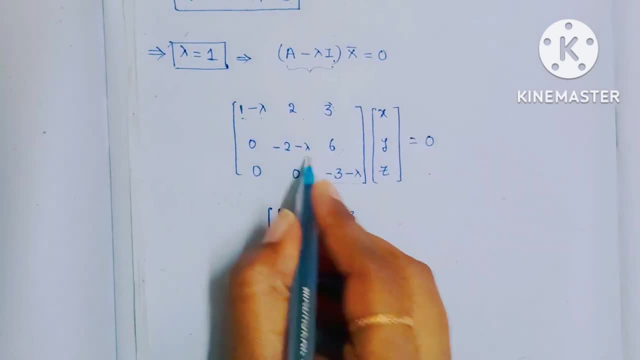 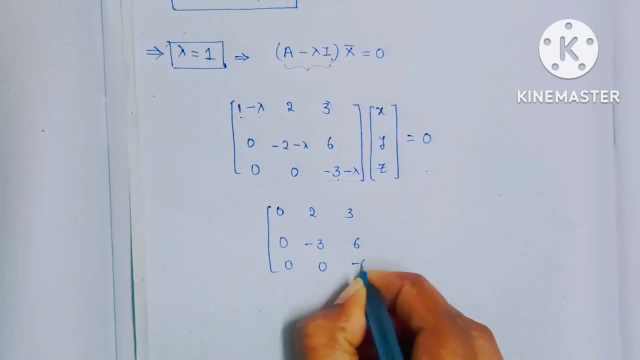 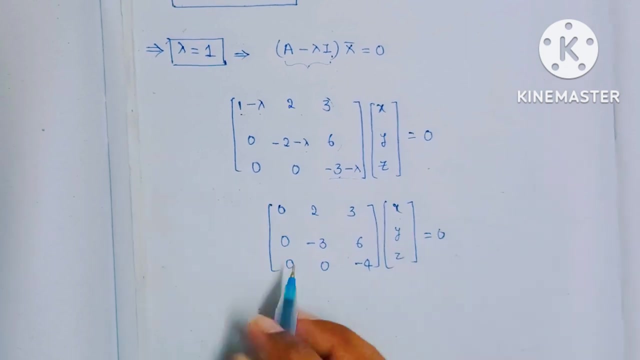 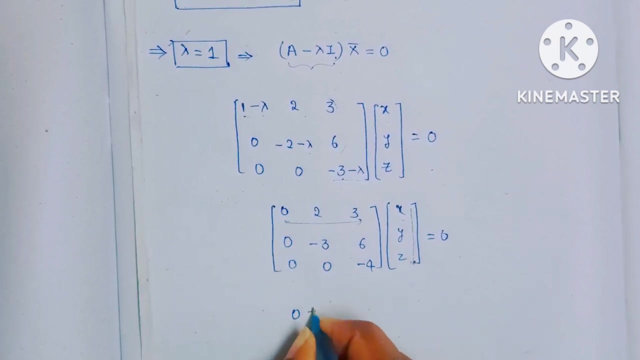 Okay, 2, 3, so 0 minus 2 minus 1 minus 3, 6, 0, 0 minus 3 minus 1 minus 4. okay, into x, y, z, which is equal to 0. from here we can write that 2 x into 0, 0 plus 2, y plus 3 z, which is equal to 0. this is the one equation. 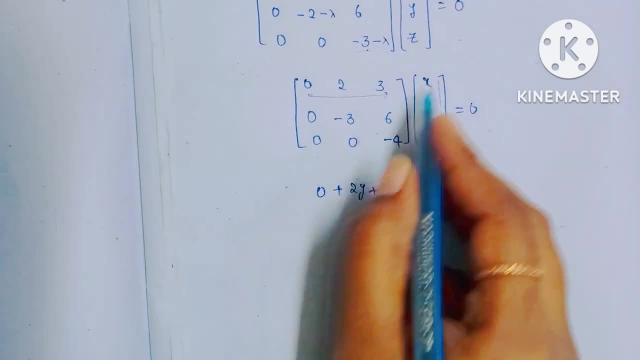 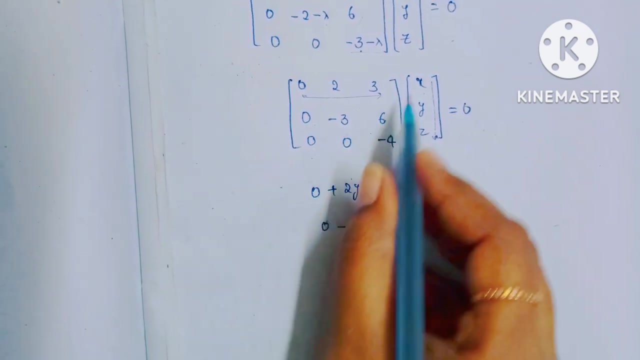 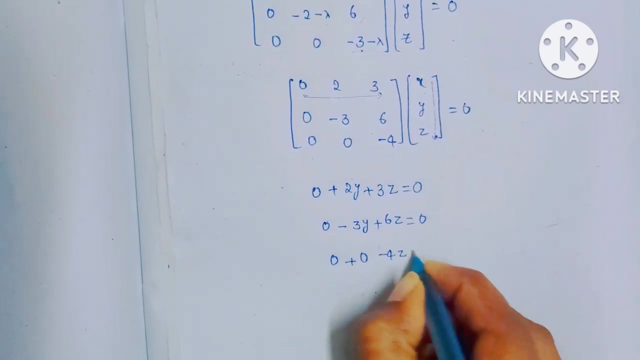 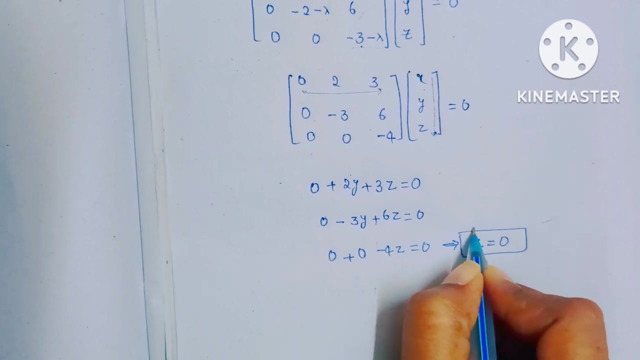 Okay, We got, and also here, 0 into x, 0, minus 3 y plus 6 z, which is equal to 0, and x into 0, 0, 0 into y, 0 and minus 4 z equal to 0. so from this equation we got the z equal to 0. by substituting z equal to 0 into these equation, we get any one of these equation. we get y equal to. 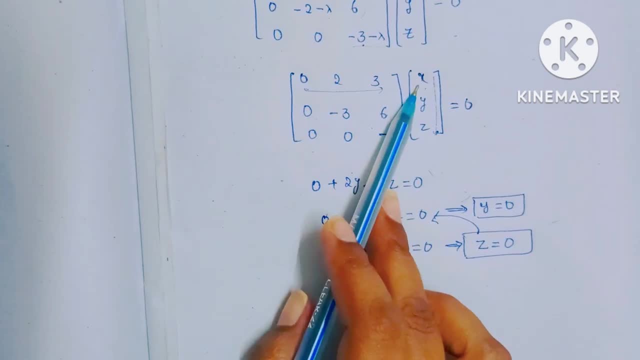 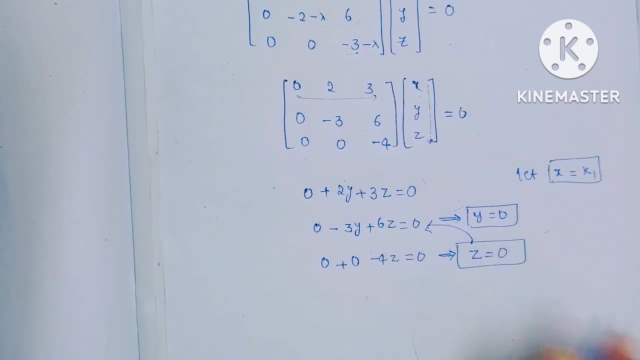 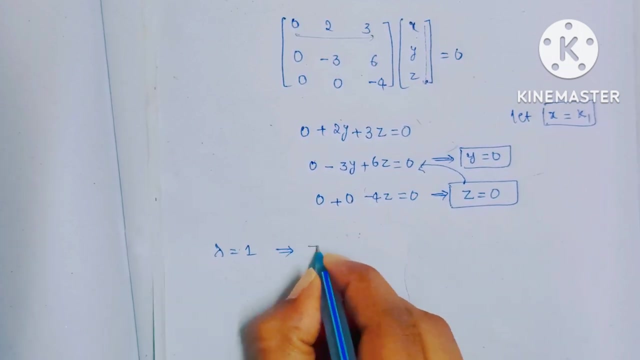 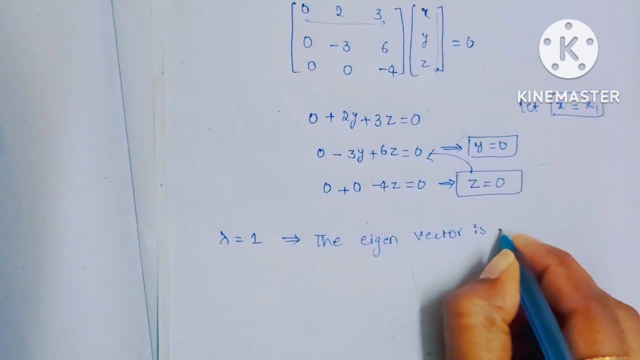 0.. 0 and also we don't know the x value now. so let we are assuming x equal to k 1. okay, so we can write: the eigenvectors is, for the lambda, equal to 1, the eigenvector is okay. the eigenvector is now that x y z, which is equal to k 1 y 0.. 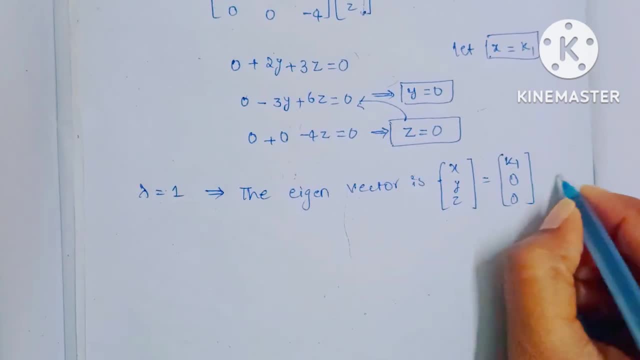 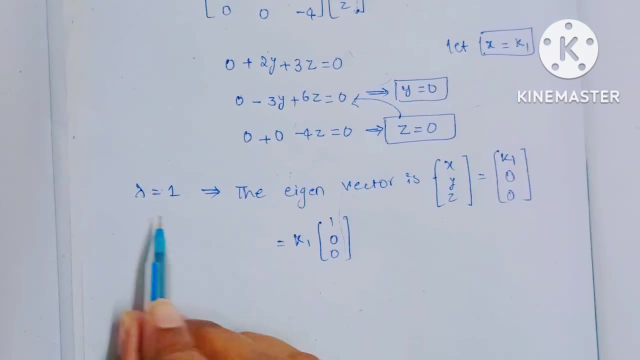 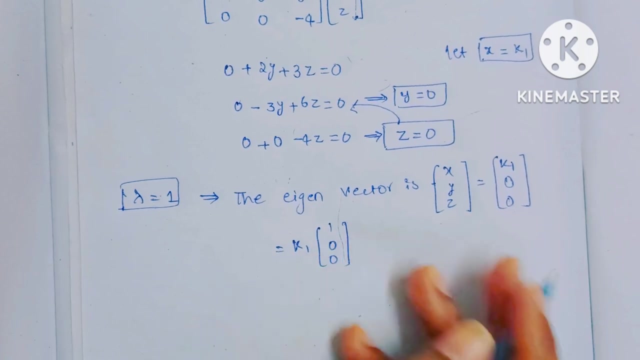 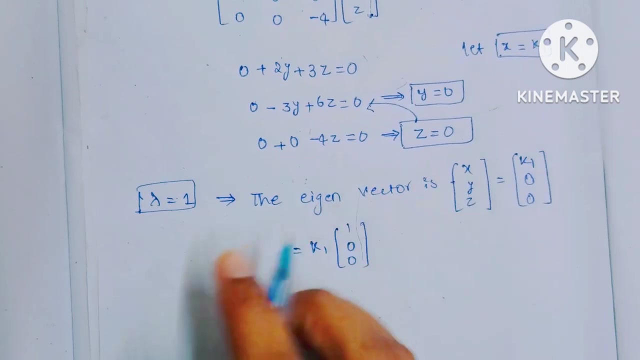 z is 0. so by taking k 1 as common we can write that 1 0 0. this is the eigenvector for the lambda equal to 1, and in comments I am observing that why you are taking k 1, k 2, k 3 like that. so I can say that here the eigenvalues are limited, that if we take n by n matrix then the eigenvalues for this matrix is: 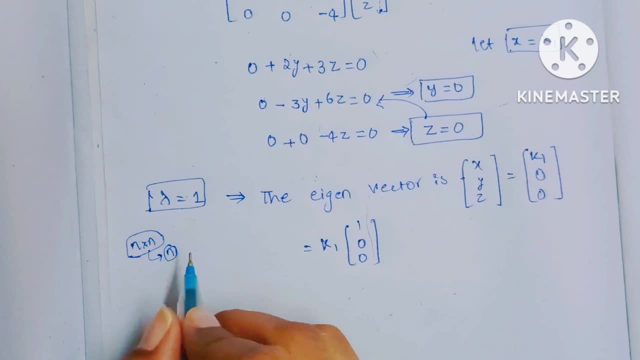 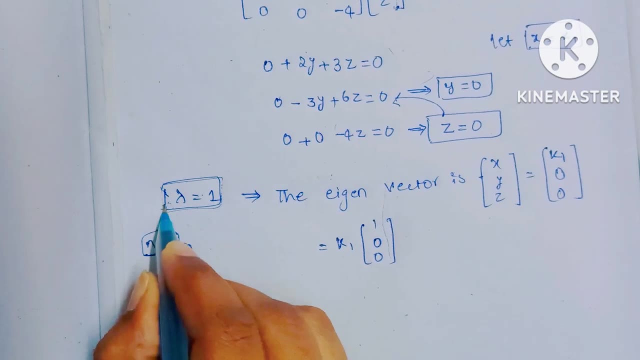 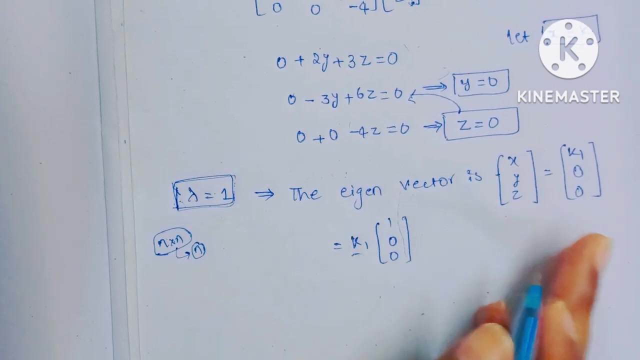 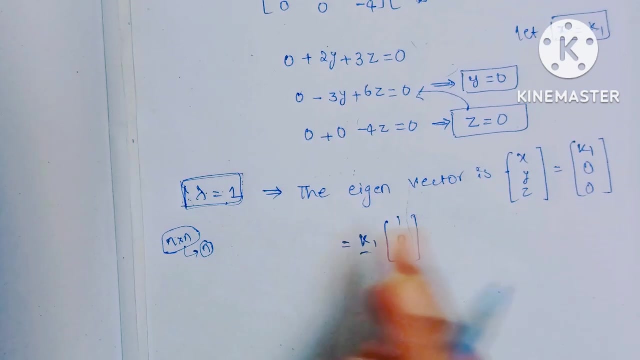 n possible. eigenvectors are, eigenvalues are possible and there is infinite number of eigenvectors will present for the given single eigenvalue, so that- so I am taking k 1 here- k 1 should be 1, 2, 3, any value. so for the lambda equal to 1 eigenvalue, for this eigenvalue there is an infinite number of eigenvectors. 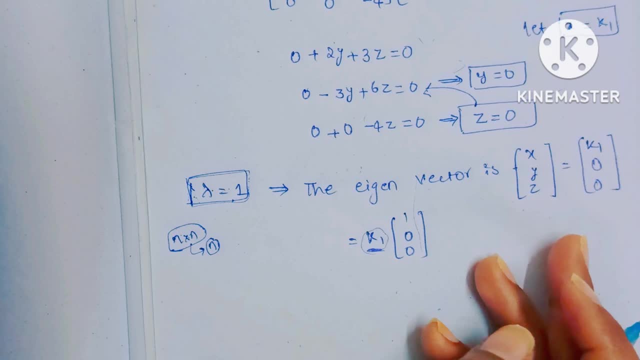 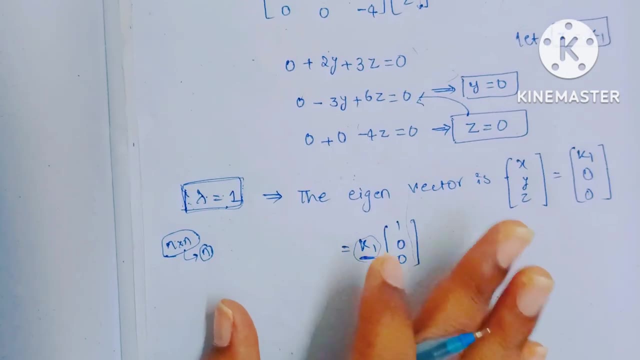 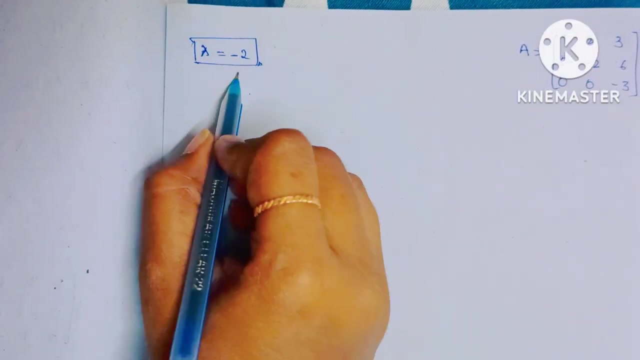 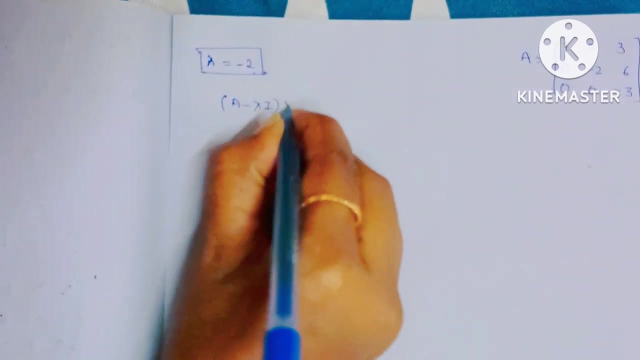 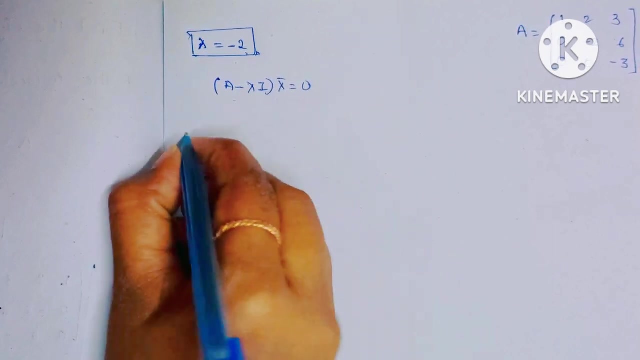 So based on this k 1 value, only That eigenvectors will be dependent. so we can write like this: also this is the correct procedure to find the eigenvectors for a given eigenvalue. so for lambda. Similarly we can find the eigenvectors for the lambda equal to minus 2. so same formula here. also a minus lambda i into x bar, which is equal to 0. so a matrix I wrote here: okay, a minus lambda into x bar. so directly I am writing here: 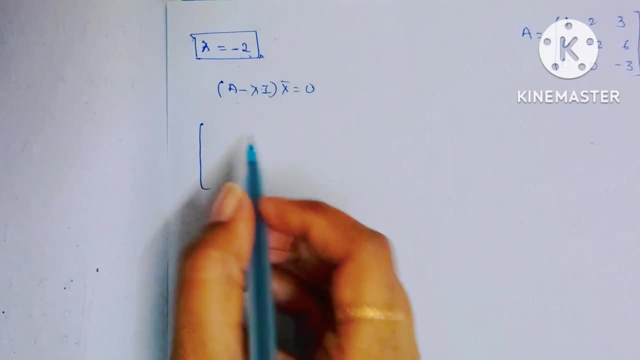 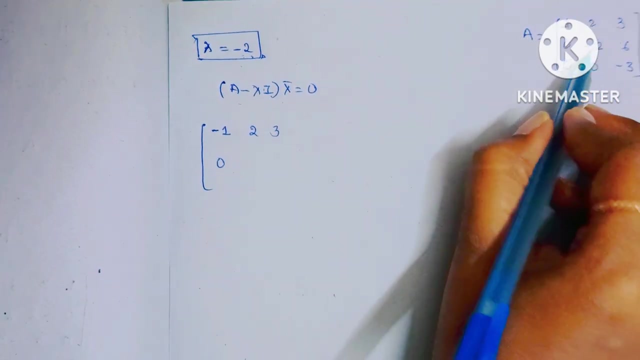 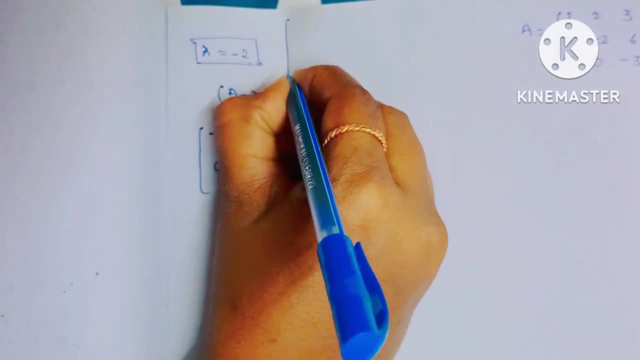 So 1 minus lambda minus 2. so 1 minus 2 is minus 1 here 2, 3. 0 minus 2 minus 2. here we get- Sorry, I will write a minus lambda i matrix here. so 1 minus lambda 2.. 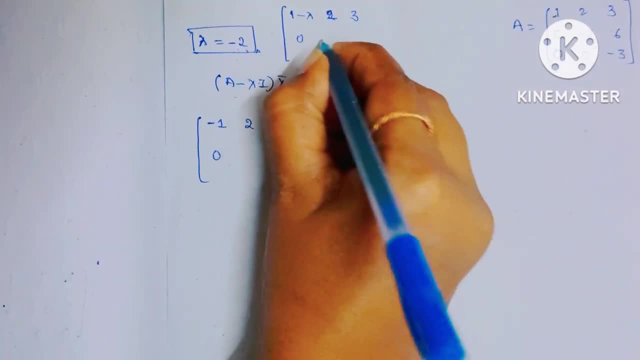 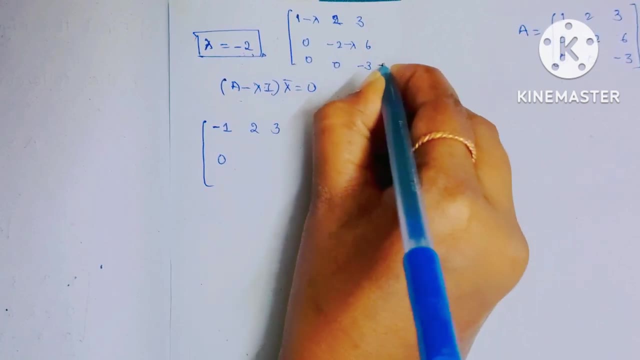 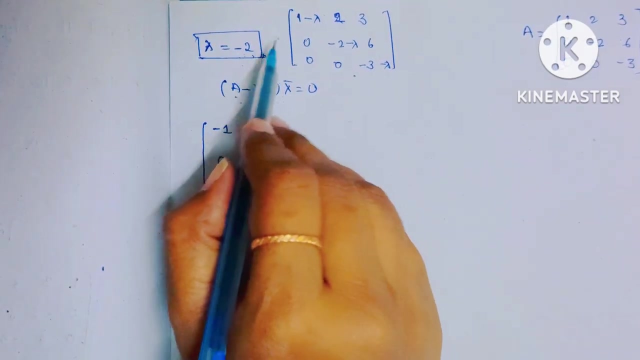 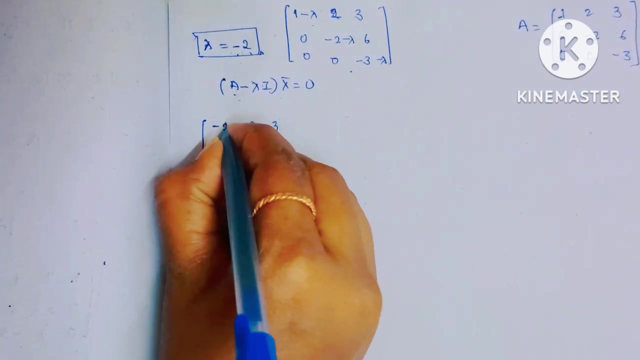 2, 3, 0 minus 2.. 2 minus lambda: 6, 0, 0 minus 3 minus lambda. This is the a minus lambda i matrix. okay, we are now. I am substituting minus 2 here, so minus into minus plus 2 now. so 1 plus 2 is nothing but 3.. 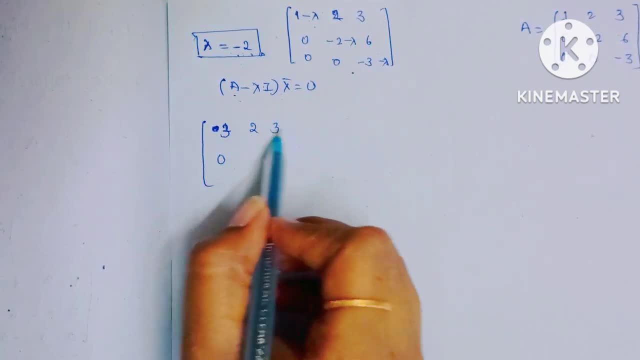 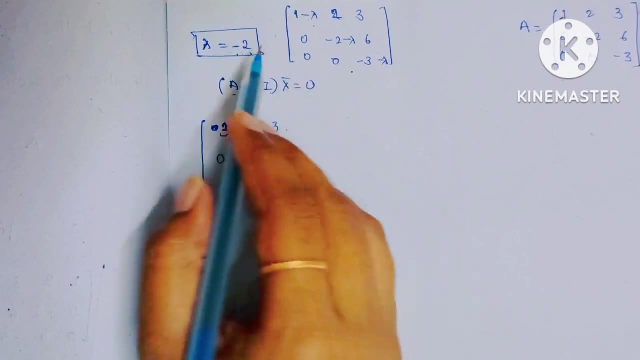 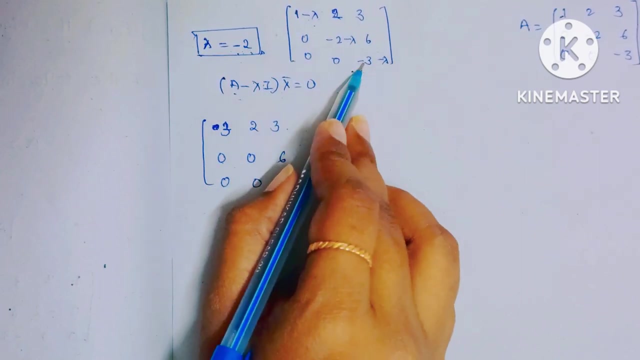 So sorry. 3 and here 2, 3 is common. and here 0, 0 and minus 2, minus of minus, plus 2.. So minus 2.. plus 2 get cancelled. 0 and here 6: 0, 0. here minus 3, minus of minus plus. so minus 3 plus 2 we get. 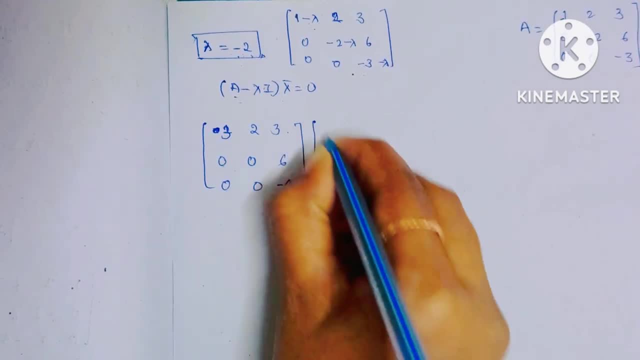 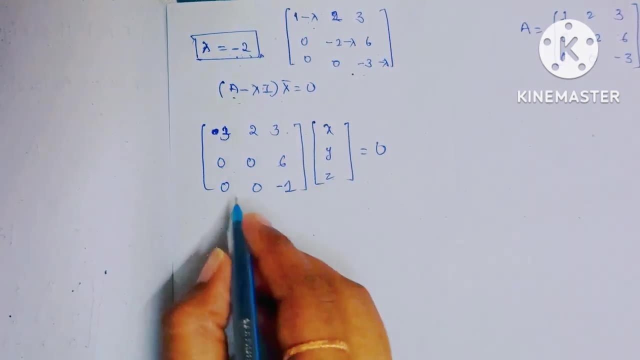 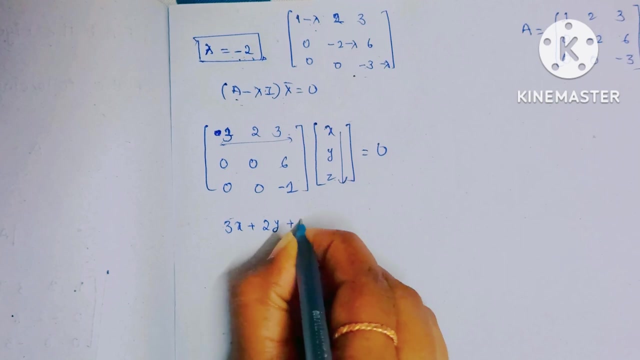 minus 1. okay, x bar is x, y, z, which is equal to 0. so from here this equation, we can write this 3 into x, 3, x plus 2, y plus 3 z, which is equal to 0. from this equation, 0 into x, 0 plus 0 into. 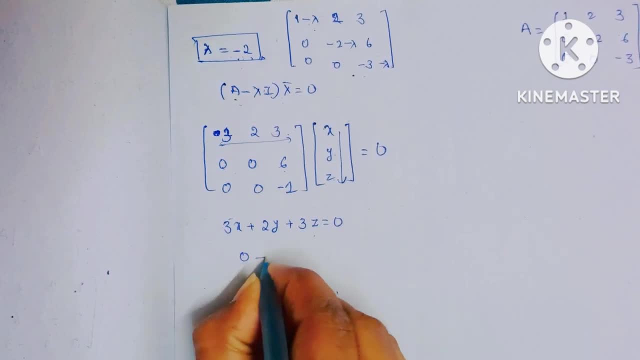 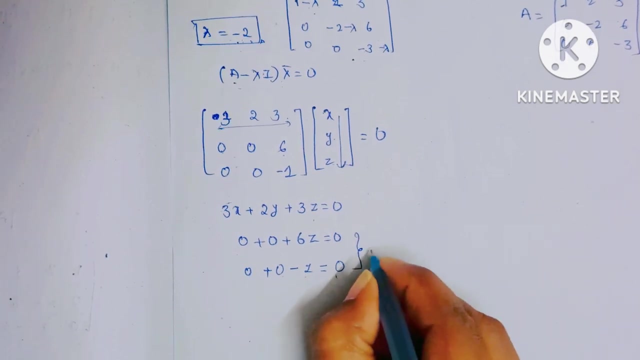 0 plus 6 into z, 6 z. 0, 0 plus 6 z, which is equal to 0. here also 0 into x, 0, 0 into y, 0 minus z. 1 into z minus z, which is equal to 0. from these two equations we can conclude that: 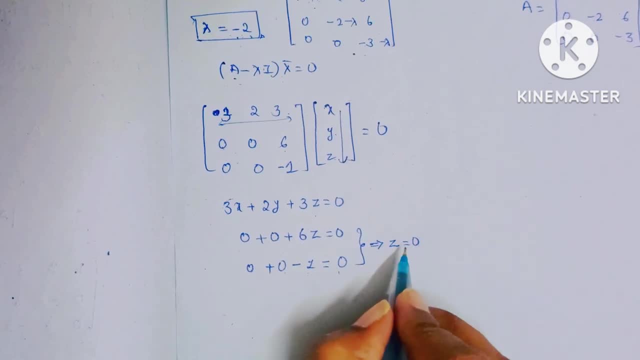 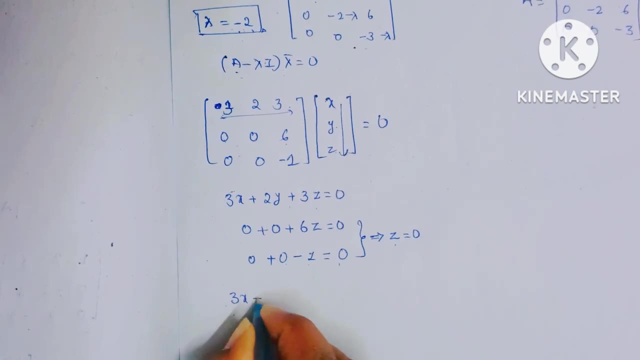 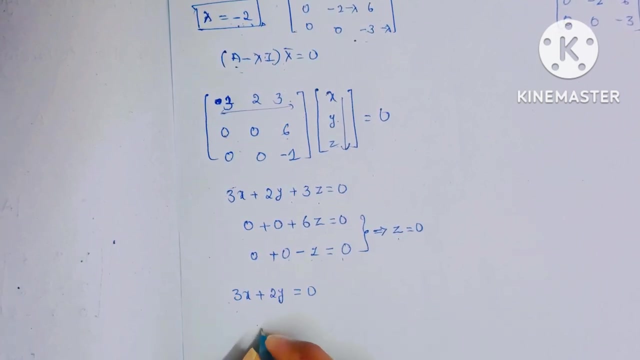 z is equal to 0.. After substituting z equal to 0 in the above equation, we get 3x plus 2y equal to 0. So we can assume x or y, anything which is equal to so let. I am assuming y equal to. 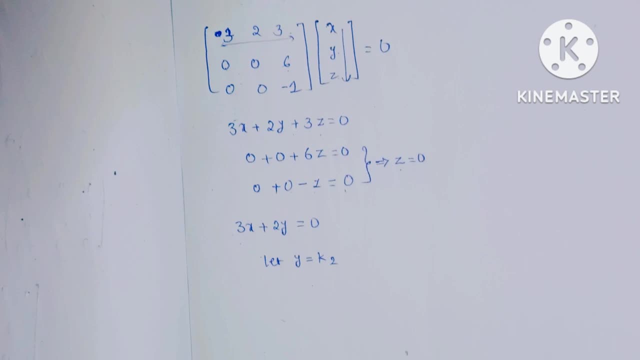 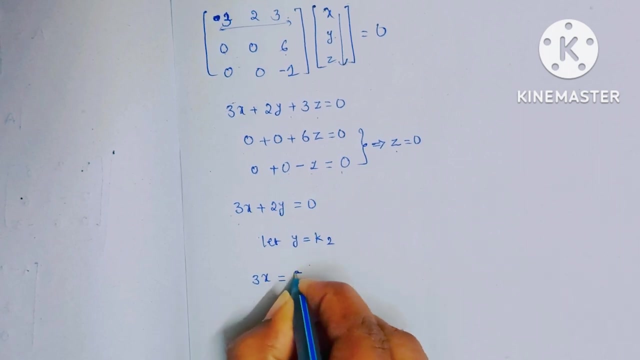 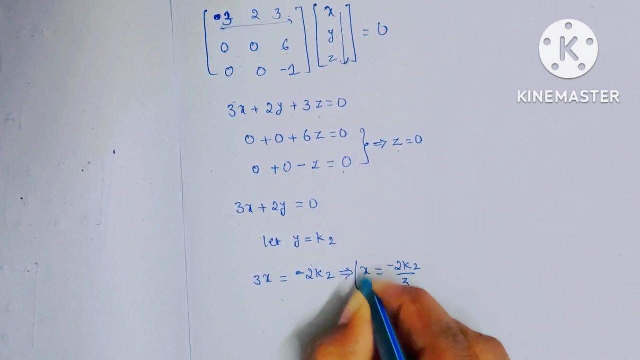 k2. ok, So by substituting y equal to k2 in this equation, we get 3x equal to minus 2k2.. So from here, x equal to minus 2k2 by 3.. This is the x value, this is the y value, and here we got. 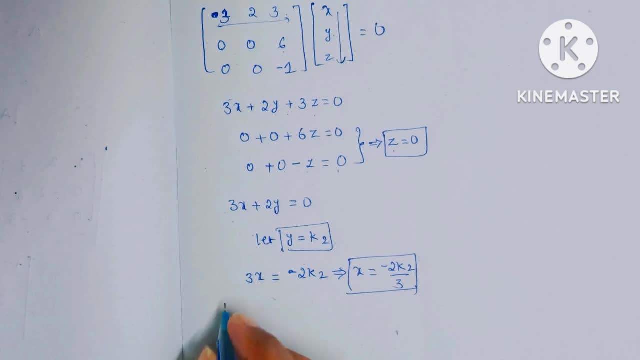 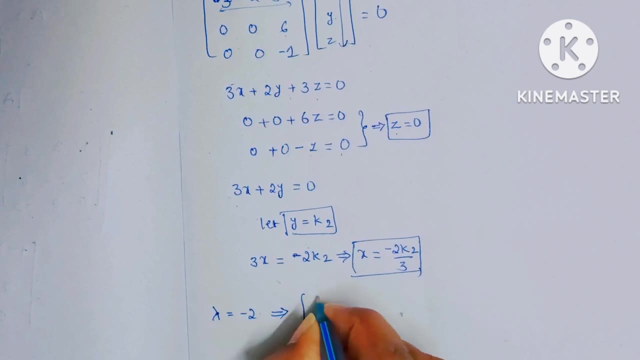 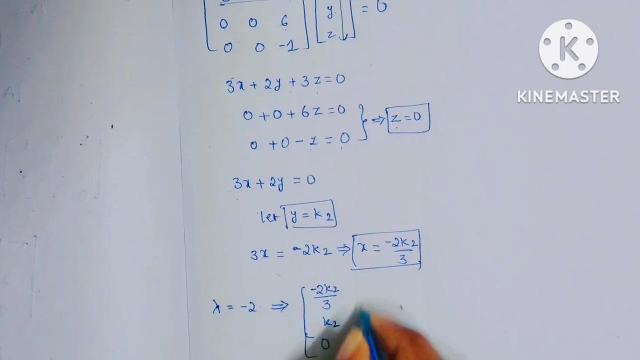 the z value. So from these three we can write for lambda equal to minus 2, the eigenvector is minus 2k2. by 3, y is k2 and z equal to 0. So this is the eigenvector By taking k2 as common. 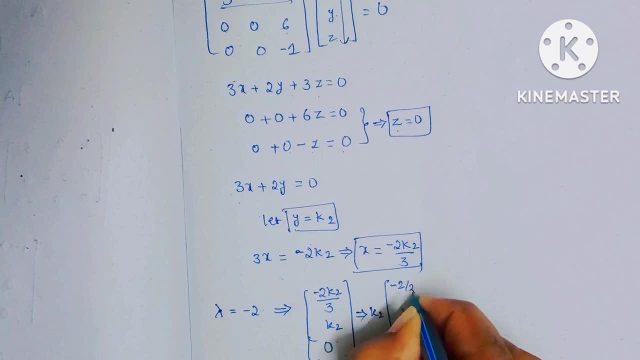 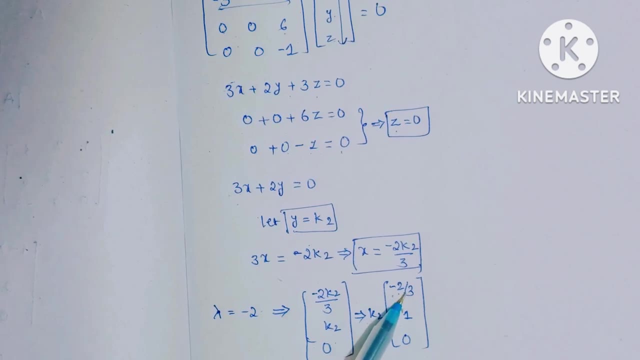 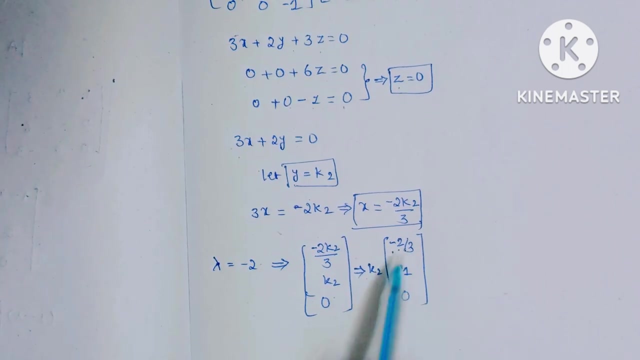 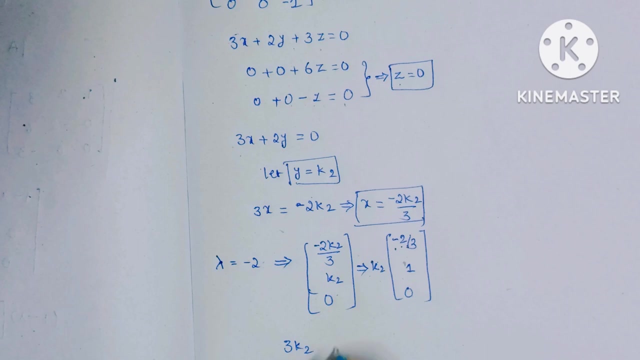 here we can write that minus 2 by 3 here 1, here 0.. If you like, if you don't want this 3 as denominator, you can take let, if you, assuming that k2 as 3.. Then we can get here, or we can take 3 common here. So here 3k2 which is equal to 3k2 into 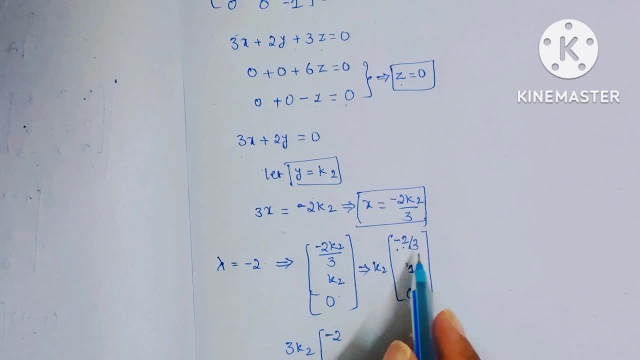 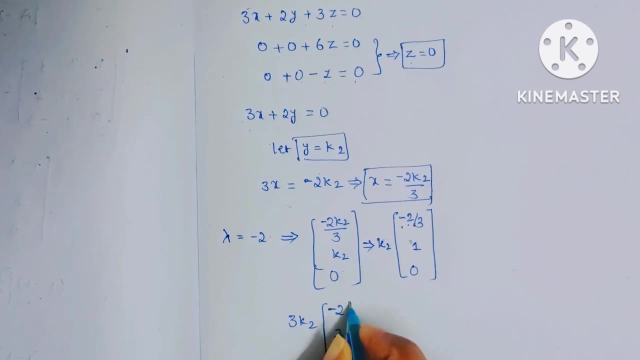 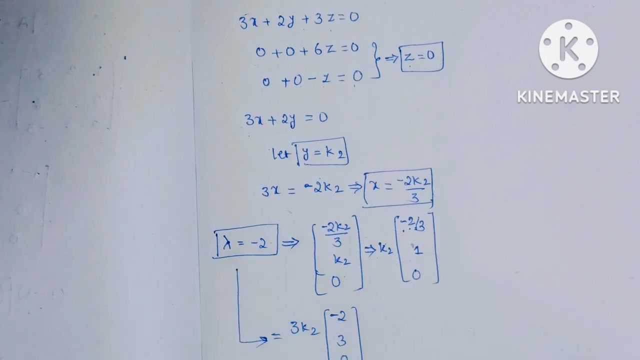 sorry, minus 2.. Here we are just multiplying with 3, that's it. So here 3, here 3 into 0: 0.. So we are getting this much. This is the eigenvector for a given eigenvalue. ok, This is the actual. 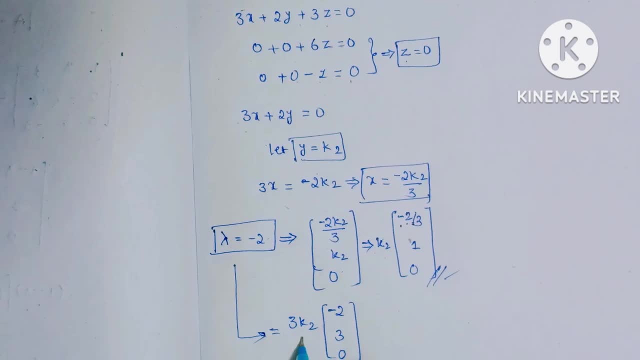 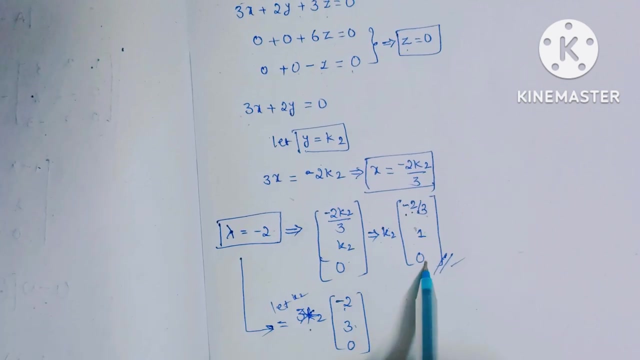 one. If we assume that k2 as 3, or if let k2 as 3. Then 3 into so k2 as 3. Then 3 into minus 2 by 3, we will get minus 2.. 3 into 1, 3. So 3 into 0, 0.. This one is the let k2 equal. 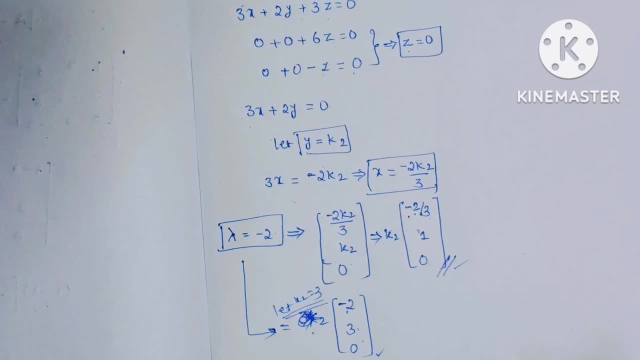 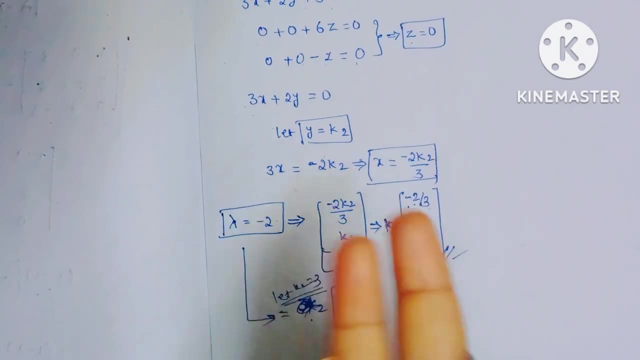 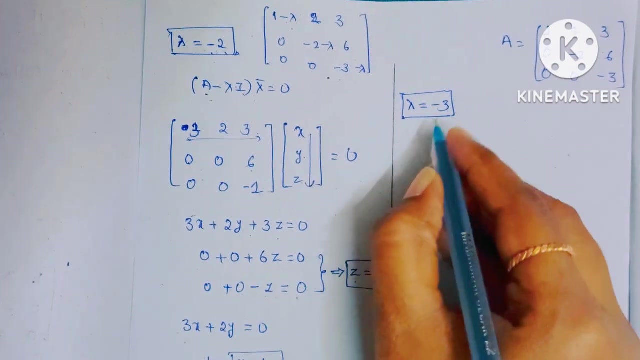 to 3.. Then only this eigenvector is possible. We can this k2 value be equal to 0. So this will be any value from 1 to infinite. Now I am going to find the eigenvector for lambda equal to minus 3.. Ok, Here, lambda equal to minus 3, we are substituting in a minus lambda. 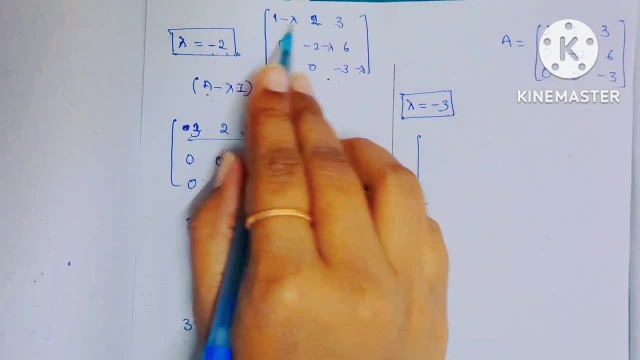 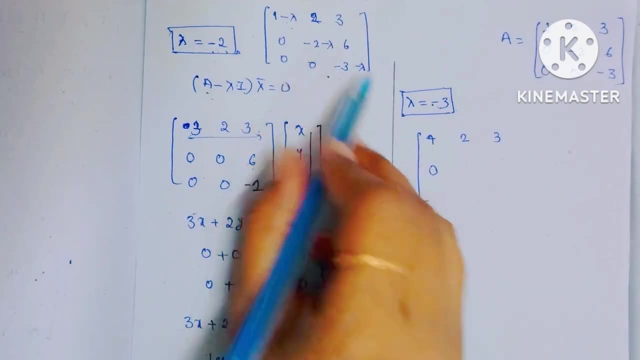 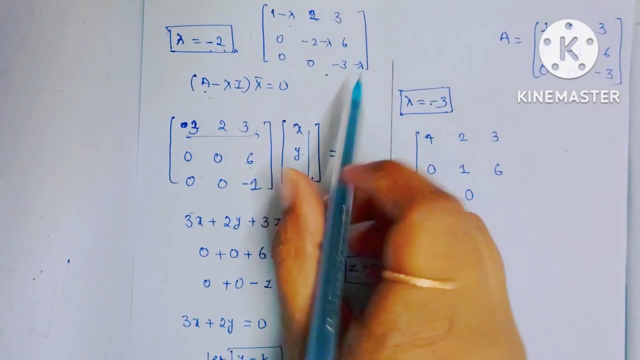 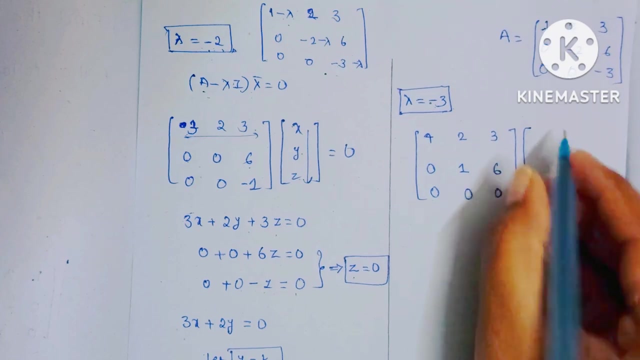 i matrix. Ok, Here we get 1 minus of minus plus 1 plus 3, 4, 2, 3 0. minus 2. minus of minus plus minus 2 plus 3.. We will get 1.. 6, 0, 0.. Minus 3 minus of minus plus 3.. Minus 3 plus 3, which is equal to 0.. And here x vector. 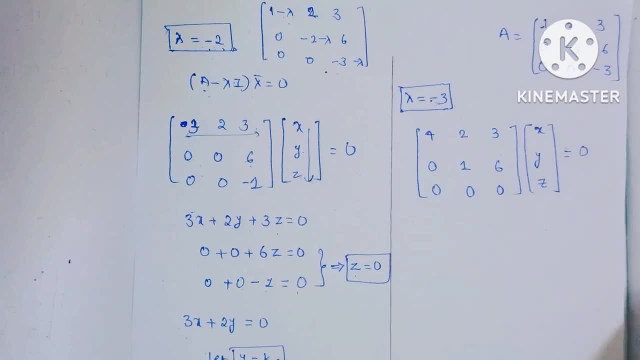 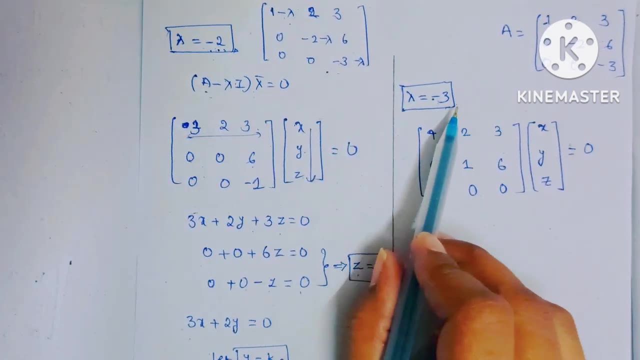 is x, y, z, which is equal to 0.. If you want, you can compare. This is the eigenvector for the lambda equal to minus 2.. And here I am finding eigenvector for lambda equal to minus 3.. You can compare. So here I am writing. 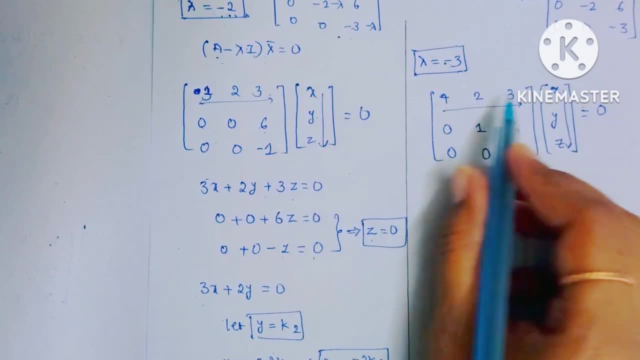 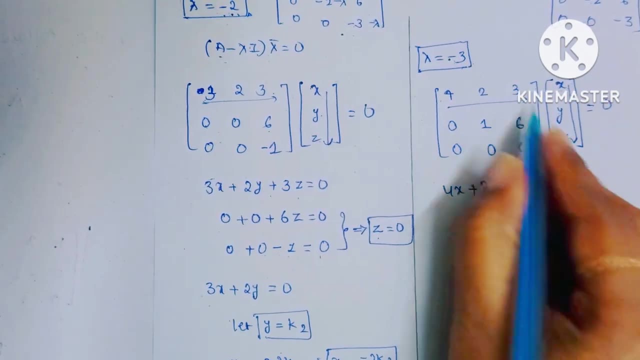 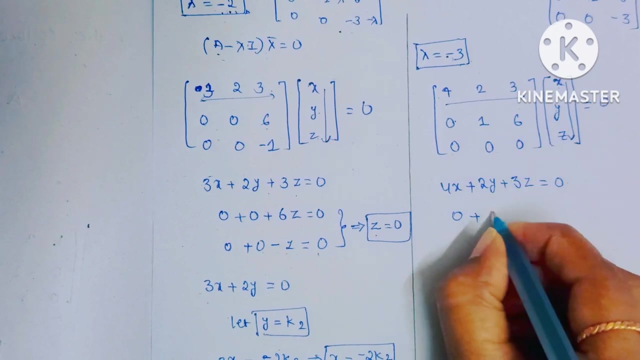 So by multiplying these 8 vectors, equate matrix 4 into x, 4, x plus 2 into y, 2, y plus 3 into z, 3 z, which is equal to 0, and here 0 into x, 0 plus 1 into y, y plus 6 into z, 6, z, which is equal to 0. 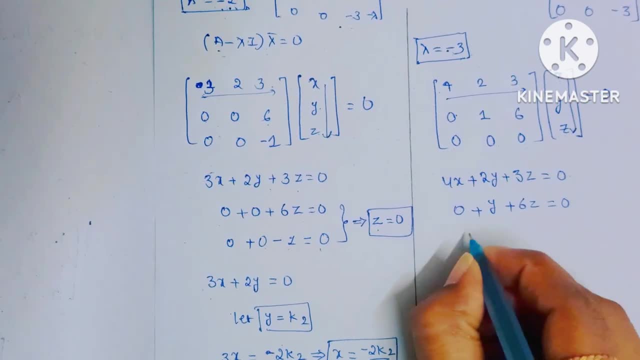 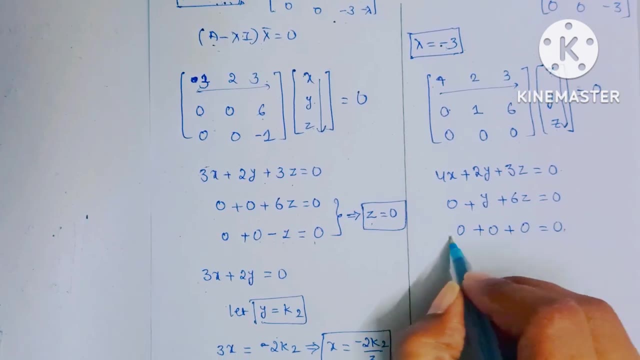 Here everything is 0, so here nothing is there: 0 into x, 0, 0 into y, 0, 0 into z: 0, which is equal to 0. this no need of to write this equation. so from these two equations, we have two equations three. 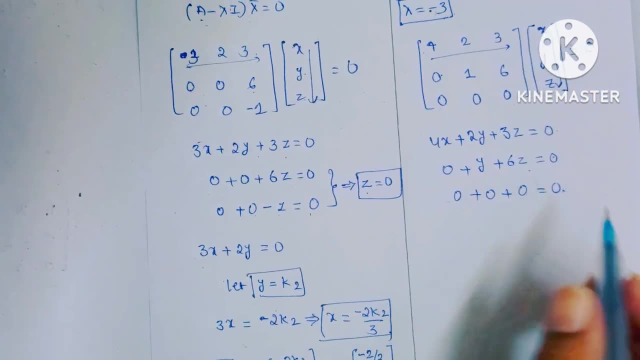 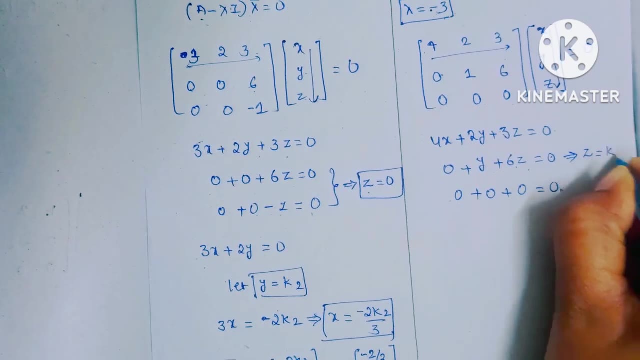 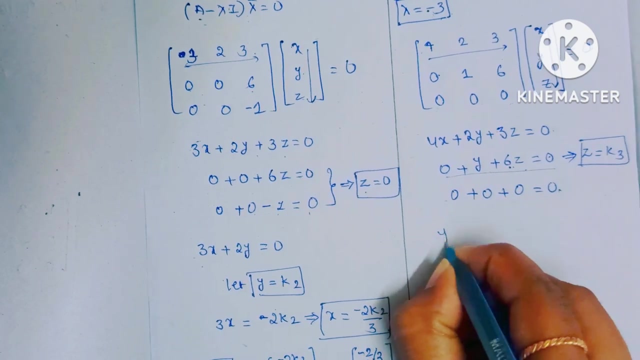 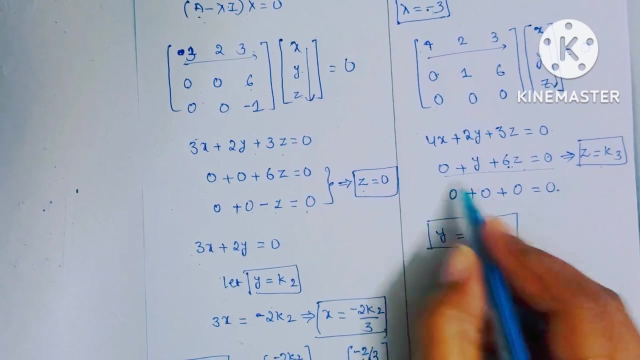 unknowns. so let we are assuming any one of value. so here we are. assuming z equal to k3. okay, z equal to k3. by substituting z equal to k3 in this equation we will get y equal to minus 6 k3. okay, and we know the z value and y value. we can find x value from this equation, so 4x plus 2 into. 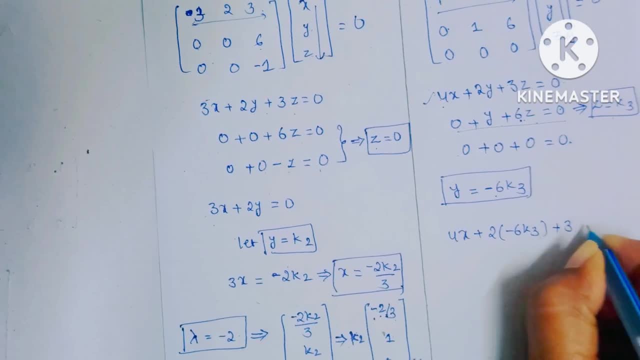 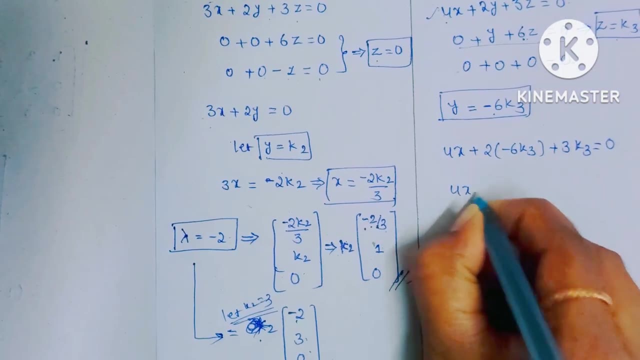 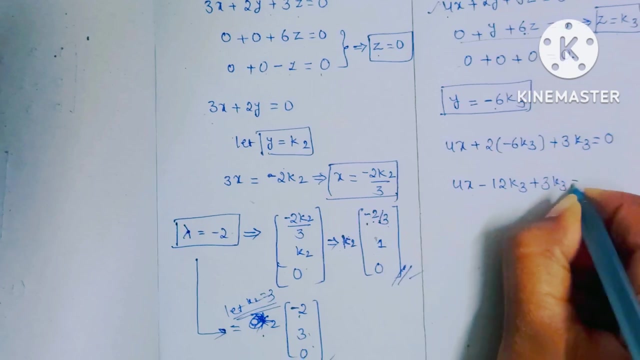 y is nothing but minus. k3 plus 3 into z is nothing but k3, which is equal to 0. and now here, 4x minus 6 to the 12, k3 plus 3, k3, which is equal to 0, 4x, which is: